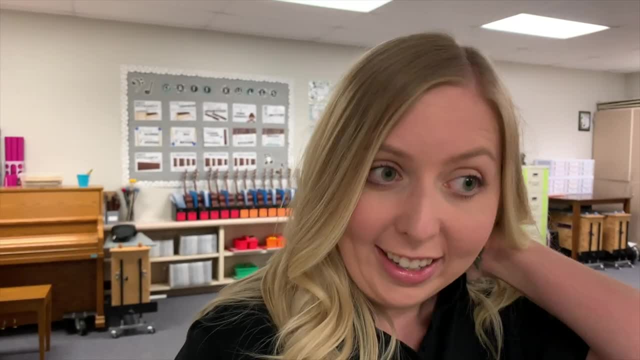 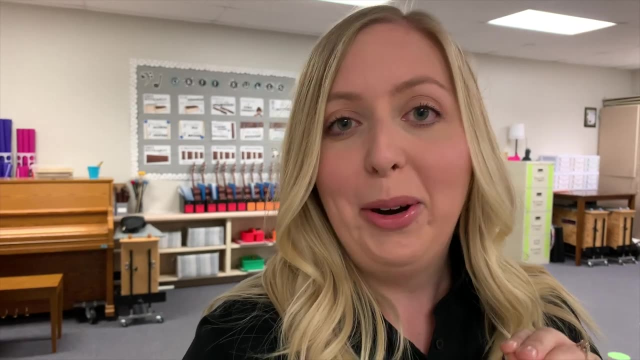 about. I can't believe we've been in school almost for three full weeks already, So I'm going to take you guys through. It's a new rotation of lessons today, So I definitely need to put my thinking cap on. I have to think extra hard on those first days, but that's okay. 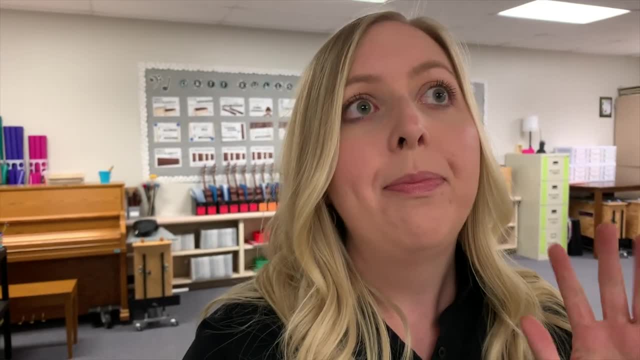 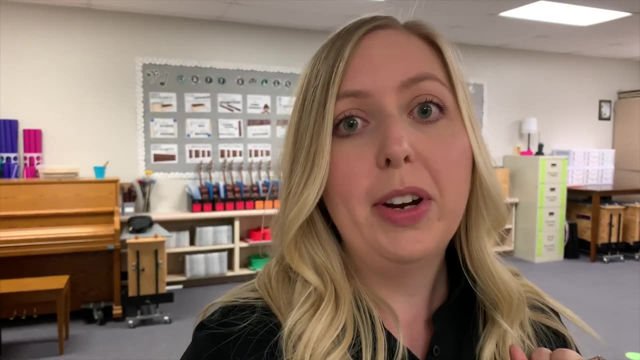 So I'm going to double check that I have everything ready for this morning. I have fifth grade, no, no, fifth grade, fourth grade, second and third this morning. So two fourth grades, one second grade and then two third grades in a row. So five classes are only 30. 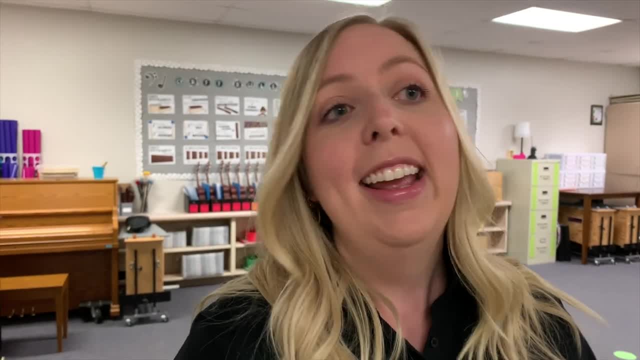 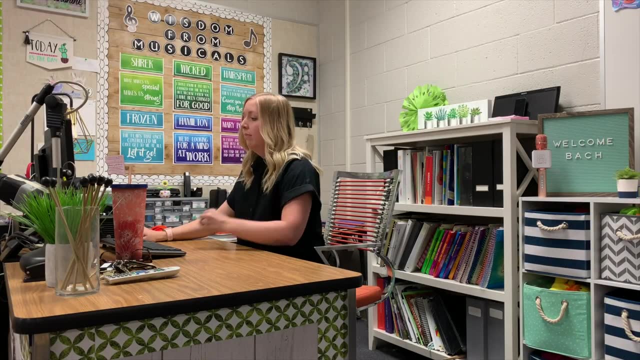 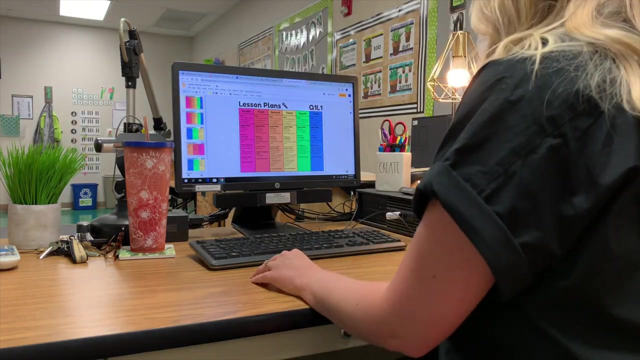 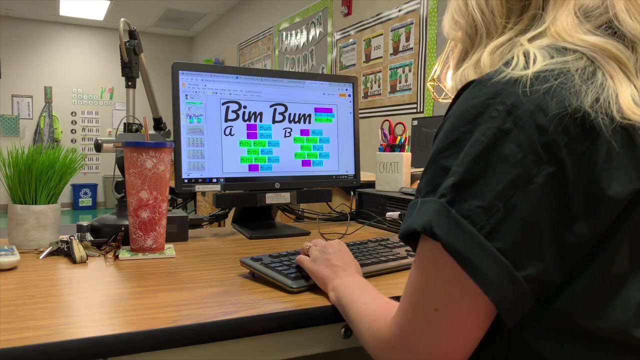 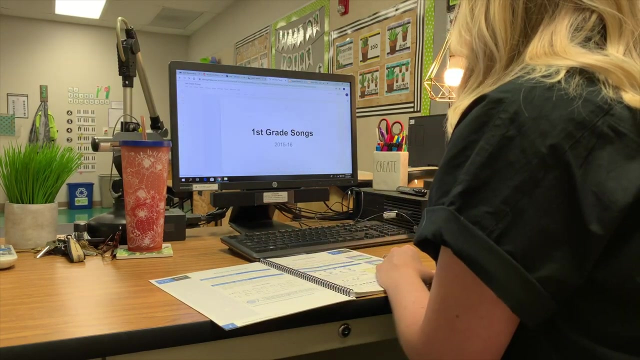 minutes, So super duper short. I have to pack a lot in there And so I will be checking in guys at lunch and let you know how it went. Young ones come crushing down. They want to feel the sun. Don't know what's in and out. They thought they'd seen the light. 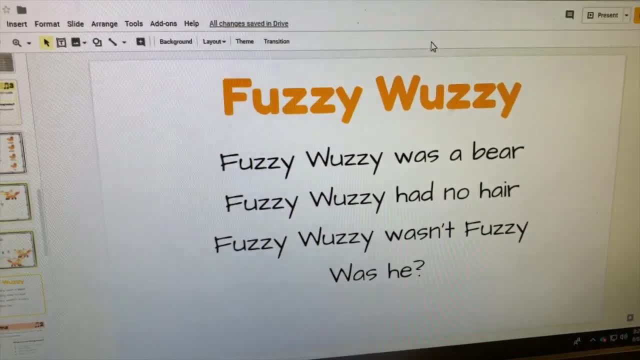 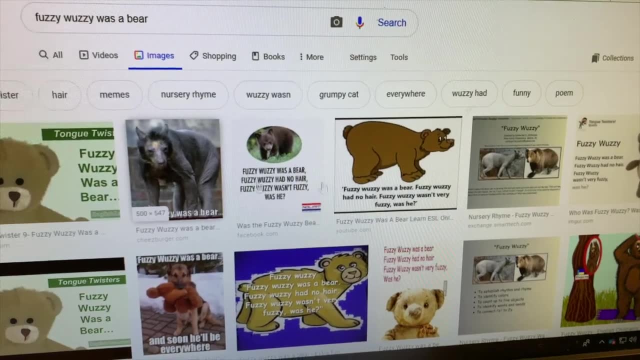 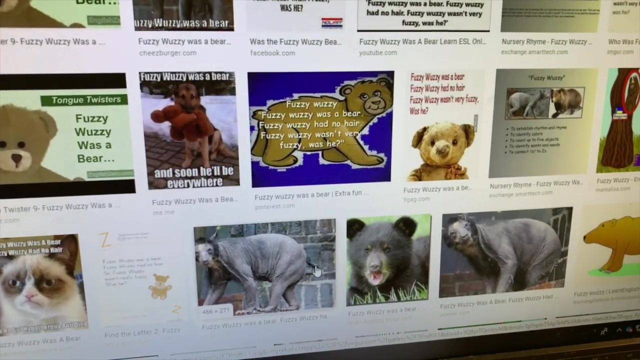 A mallet activity For fuzzy wuzzy this morning And, um, I searched- fuzzy wuzzy was a bear- and for the images. And this is frightening, Like what. I can't even put that on there. That is so frightening. I'm just going to go with a normal bear with hair, because that looks like it should be in a horror film. 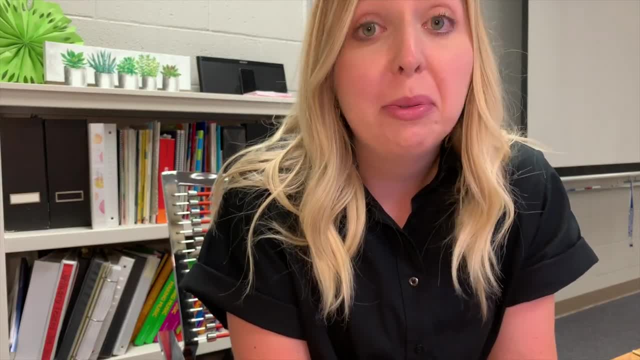 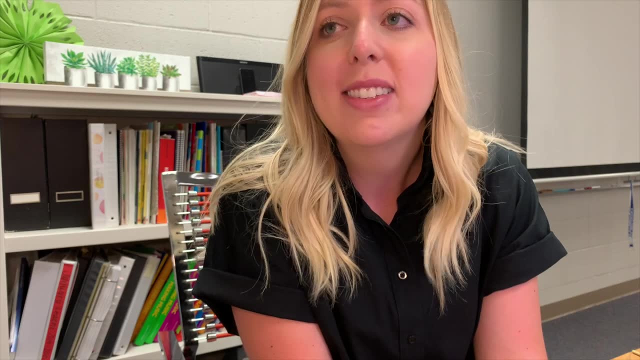 Okay, So I am done with my morning classes. They all went really well. Actually, it just is a little chattiness, but that's just. we should be doing it to be expected The third week of school. kids, just you know, are not in those. 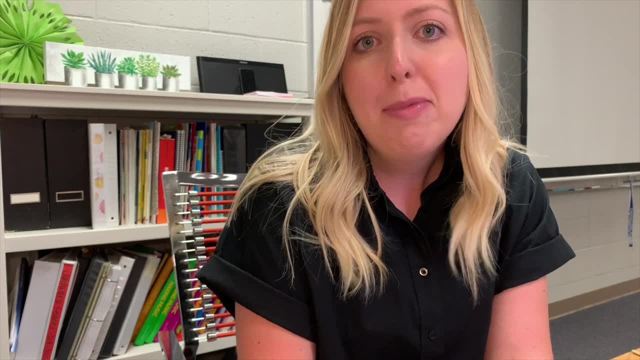 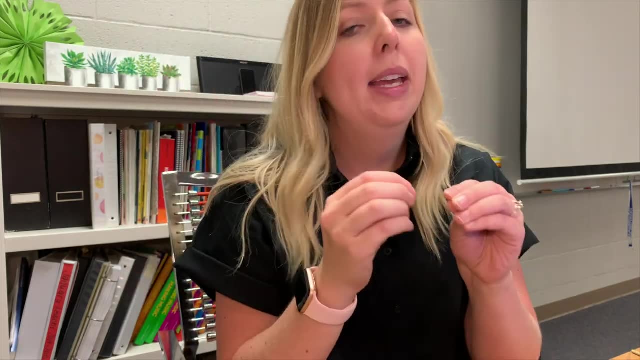 routines. Um, so, a lot of that. it's definitely pick your battles, but, um, yeah, so I definitely need to go back and make sure, like the next round of classes, that I'm really nitpicking at that, Because if you know, as you know, as a teacher like you, let that go for now it's going to be. 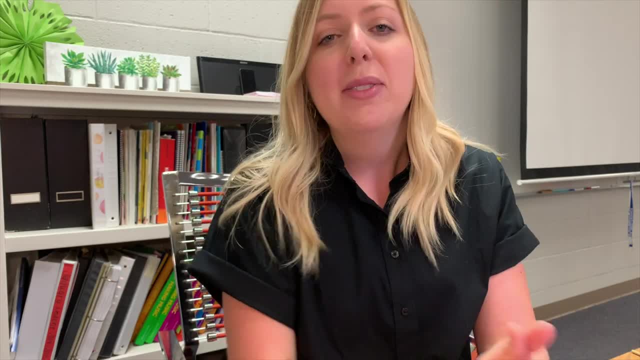 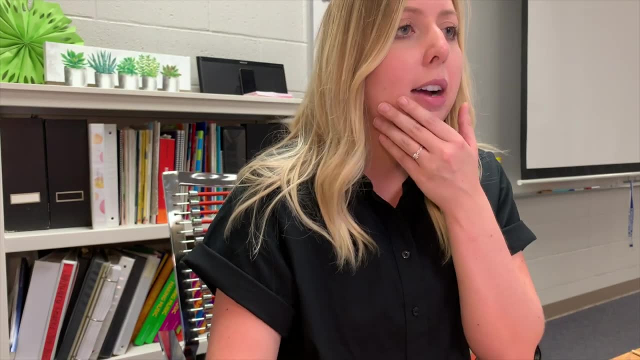 way worse later on. So it's kind of manageable right now. So I am going to definitely be reminding them a lot more about that. Um, but my lessons went really well. me kind of break down what I did, So let's see for fourth grade I do this clapping game, the. 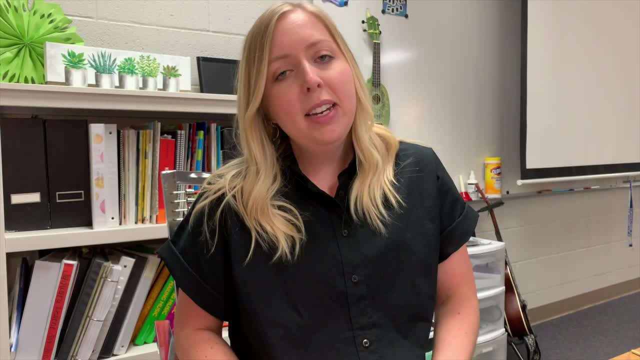 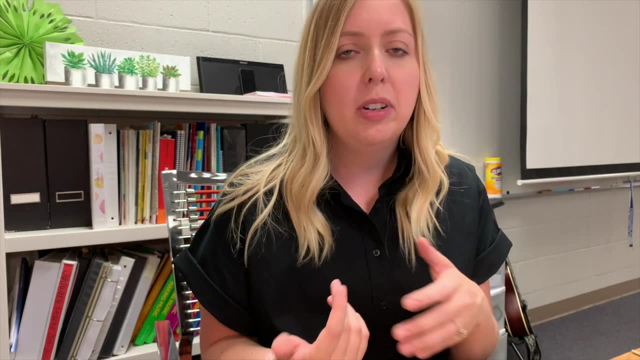 classic clapping game: bim bum, bim bum, bitty, bitty bum, bitty bum, bitty, bitty bum, bim bum. So if you have ever heard of that, it's a really well-known clapping clapping game. If you just 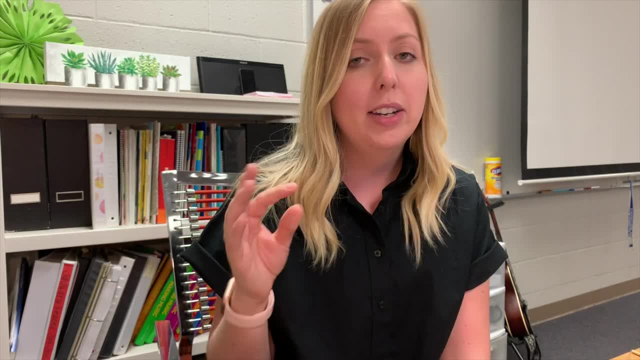 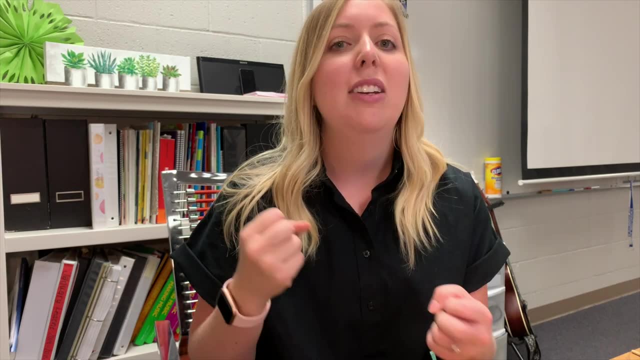 put bim bum and YouTube, you will see it. So I am teaching slowly that to fourth grade. Last lesson I taught them the first half and then I taught them the second half. today And as soon as I say like, like you know, we're trying to get as fast as possible and kind of make that competition part. 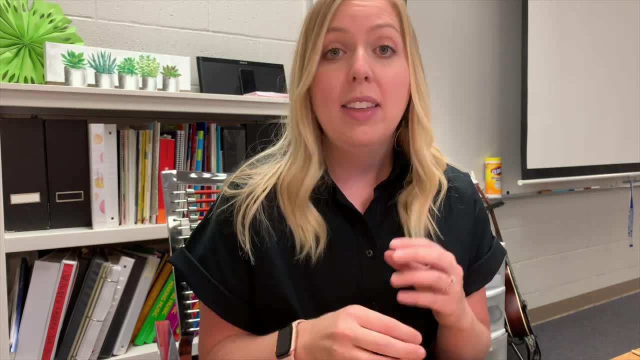 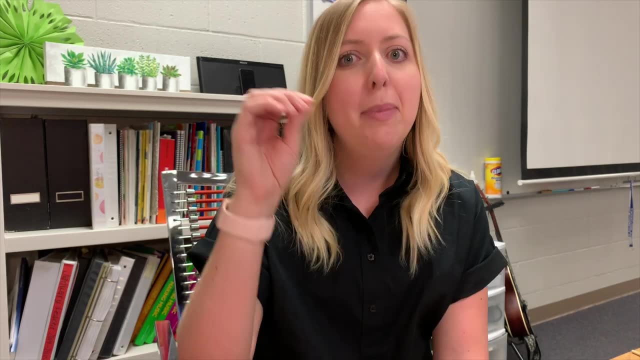 I really hook them and they really like it, So we're going to do that. And then I have actually a group project that I do with them where they change the three words. So there's bim, bum and bitty, And so they change each three words to something else, So it might be like grilled. 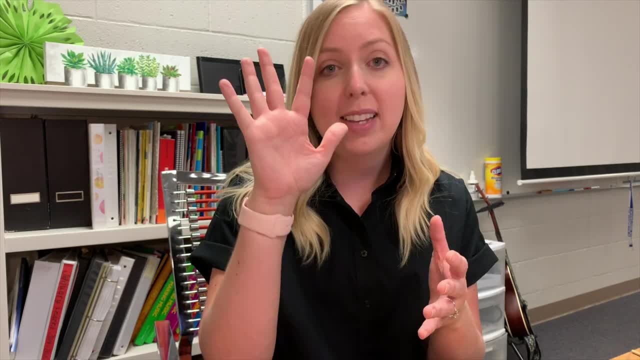 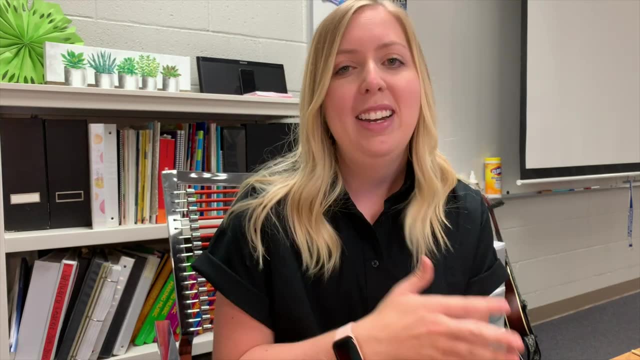 cheese yum, And so they have to change that order. It's the same pattern, but they have different words now And then they also can change the movement. So that's a project that we do, But right now I'm just teaching the original version. We did apple tree to um to review. 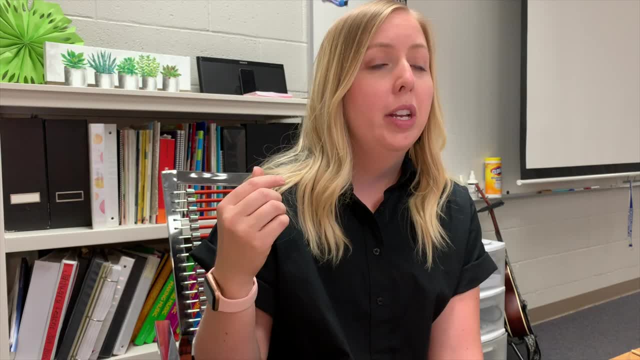 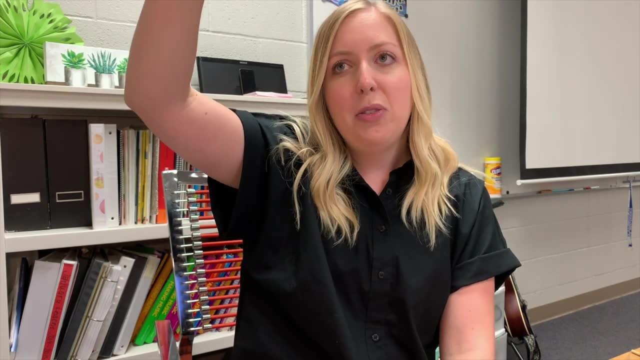 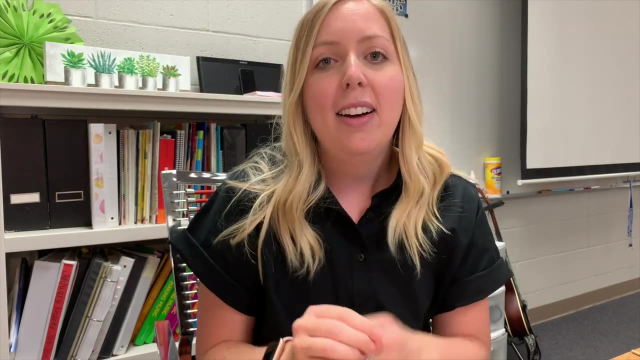 low dough And so we played the apple tree game. I do it, the version where they walk around in a circle and you have one person holding a bean bag over top And if you are on out you are standing underneath someone with a bean bag. you drop the apple, you tap them on the head. they got knocked. 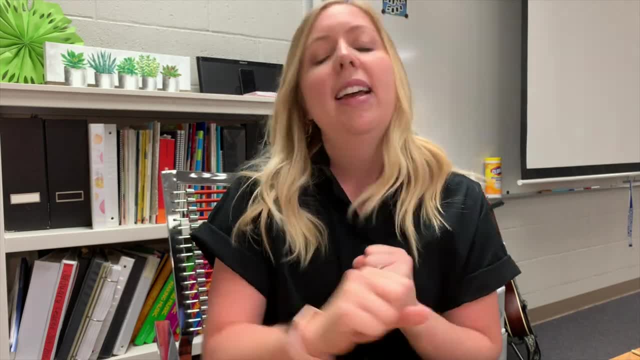 out, and then they're in a tree with you, And so there's just more and more trees and more and more people that get out of the tree, And so that's what we do, And then we have a group project that gets out, and I usually don't go to just one winner at the end, because it's just too chaotic. So 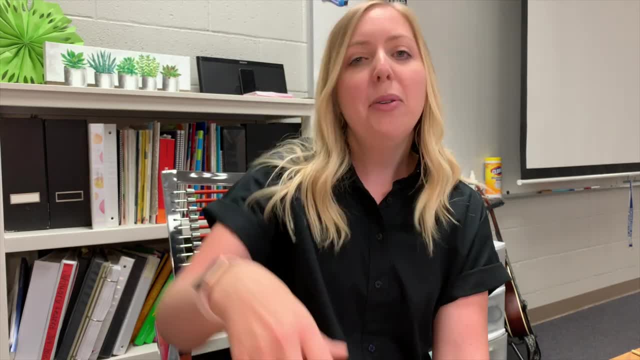 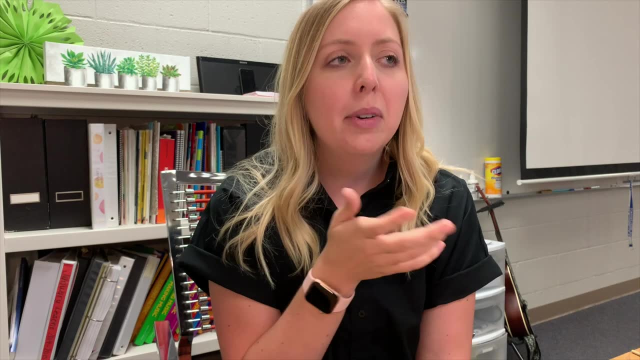 once I get about maybe seven ish students, I say, okay, you're the winners and we're moving on because it's just a little too difficult. And then also I do this Pokemon game, So I'm created. I'll have to see. I really want to make like some way that I can have you guys get access. 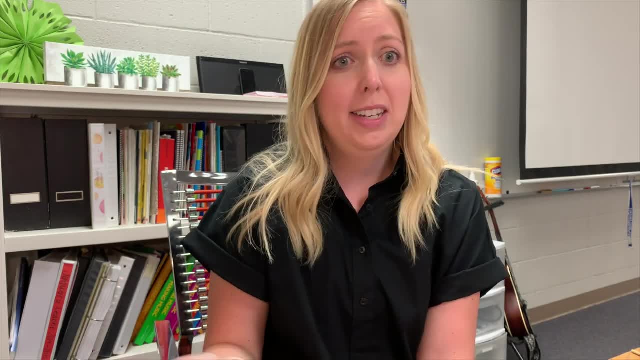 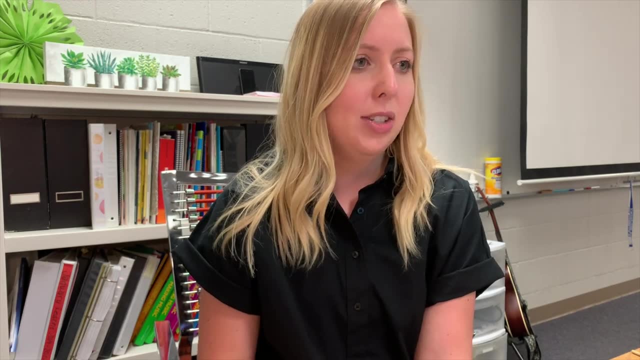 to some of some things that I can't really sell on TPT because it's copyrighted materials. Like, I have a lot of Pokemon clip art, you know, just for educational use, And so I will see what I can do because I want you guys to have access to that. You know it didn't why. why would I just 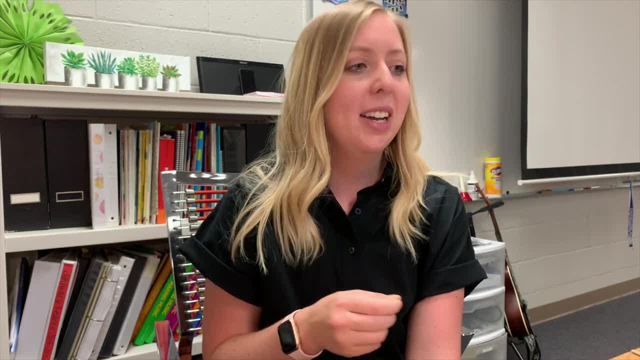 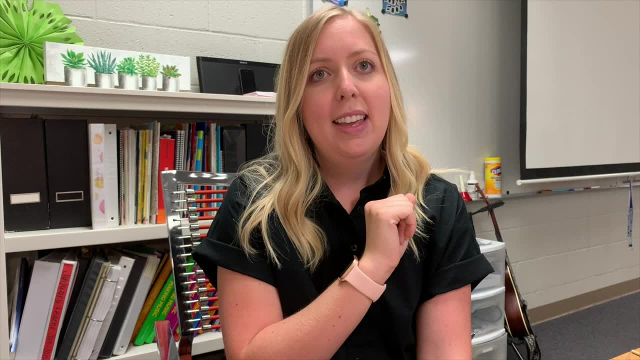 keep it to myself, You know. So I will see if I can figure that out. but it's pretty much a dictation game. So they try and catch the Pokemon. they pick one to catch and then they have to listen to. I have, like, already prerecorded a rhythm that I play on the cowbell, And then they 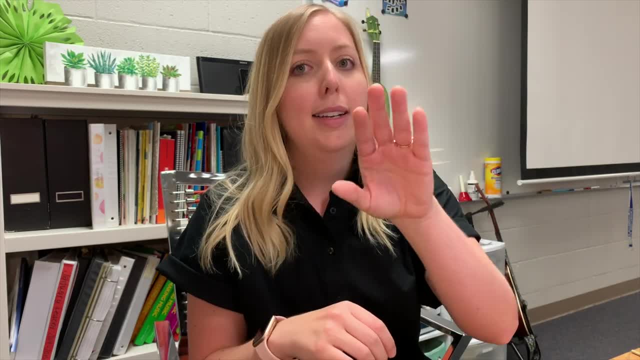 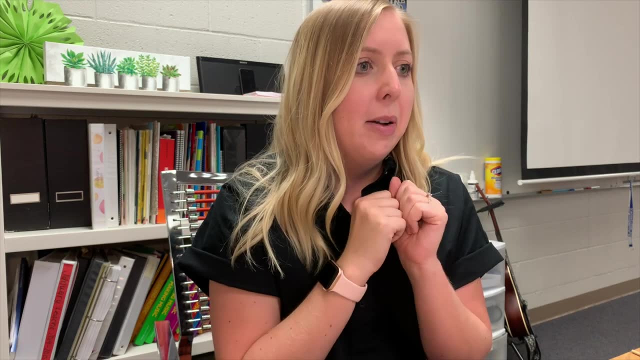 have to figure out which Pokeball it is, So like ta ta, ticka, ticka ta or T T, T T, ticka, ticka ta. They have three options and they have to pick Right Pokeball to catch it. Um then, third grade, I did chicken on a fence post which is just like: 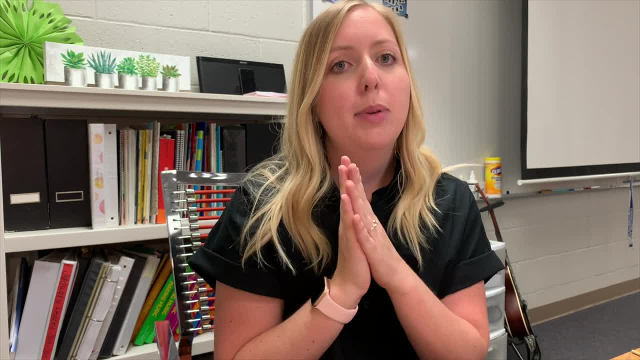 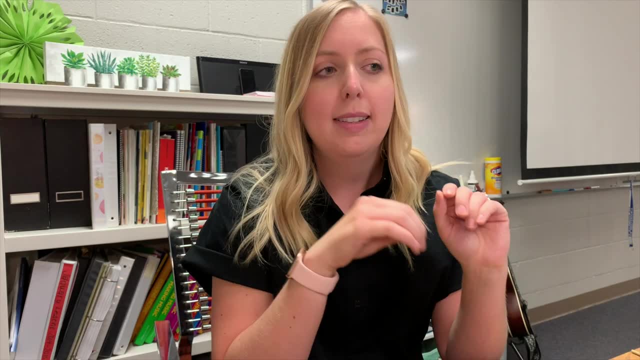 my favorite game ever. They really love it. I would just say, with chicken on a fence post. If you, when you do that, just make sure you have a visual of how the game works, because I have taught it a few years back and it wasn't as successful because it was so hard to explain what you're. 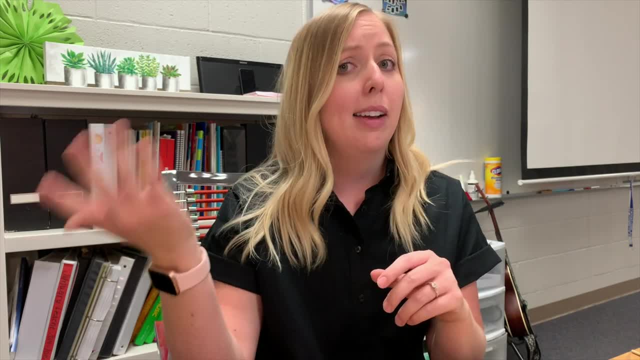 supposed to do, But as soon as I showed a visual or picture, I think I got like a file off a teacher- being teachers, and they had a visual of it. It was so easy, They got it right away and we could have fun. 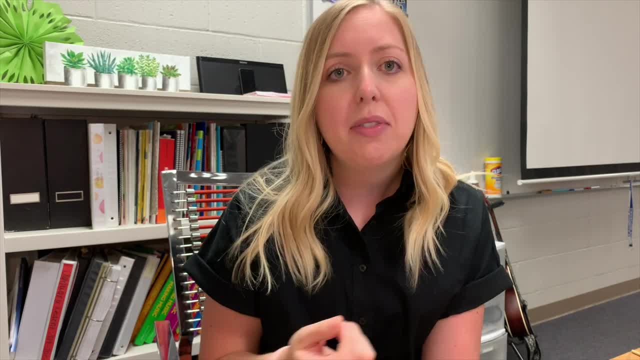 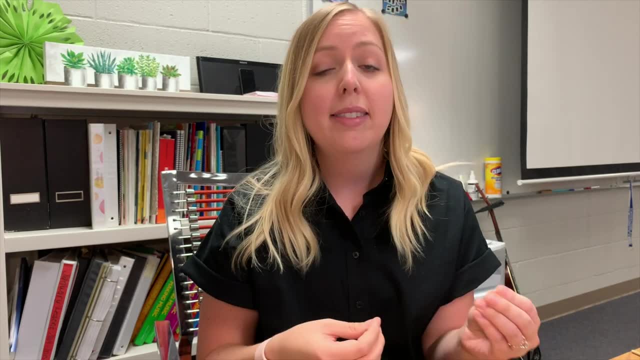 And then I also did fuzzy wuzzy. That's out of game plan. So if you've never heard of game plan, it's an awesome like kind of Orff movement. um, you know, Kodai based uh curriculum And they have a lot. 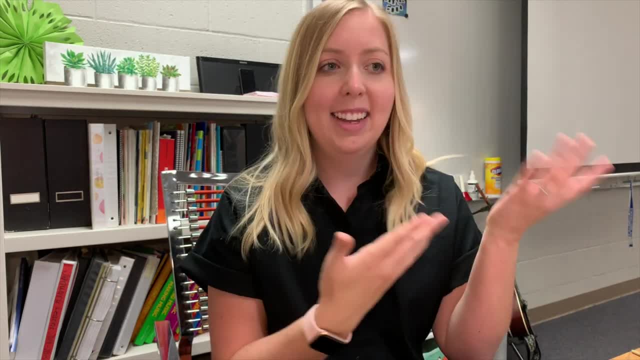 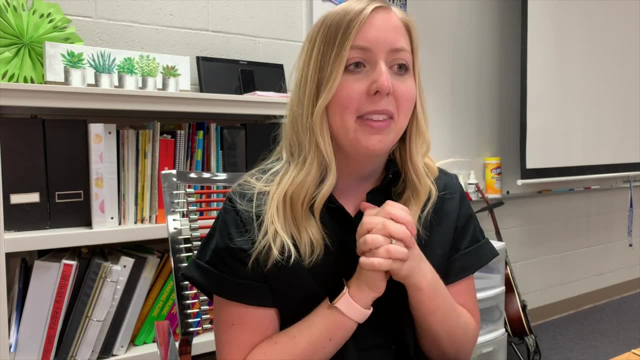 of really good instrument pieces in there, And one of them is fuzzy wuzzy. as I was looking this morning for a clip art for that And I just used a little cute bear instead of the hairless bear there, Um, but I taught them the rhyme and then they have to play on every fuzzy wuzzy two mouths. 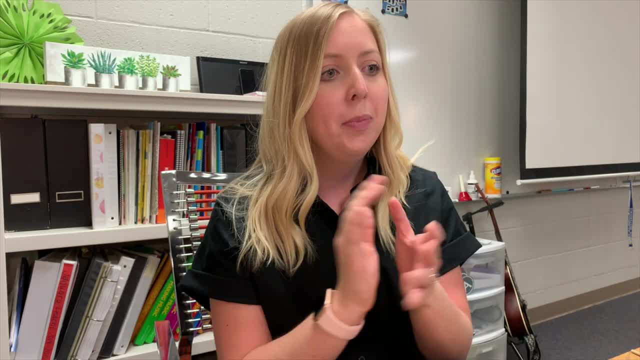 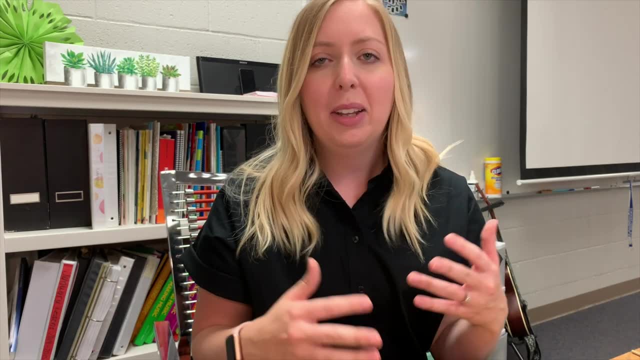 together And then I added a little drum beat and always, every time I add a drum beat, it's crazy how much kids are all like whoa, like we really made music, Like they're like, wow, Like, and so it's just really cool. I have to remind. 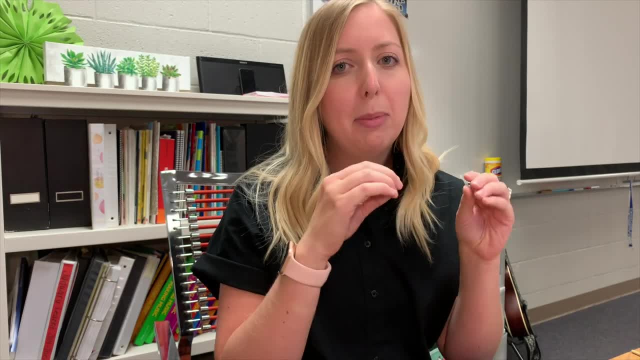 myself like I need to do that. I want them to be successful first and be able to do it without the drum Cause you know, once you add another part it starts to throw them off. They're not quite as sure, but I did a. 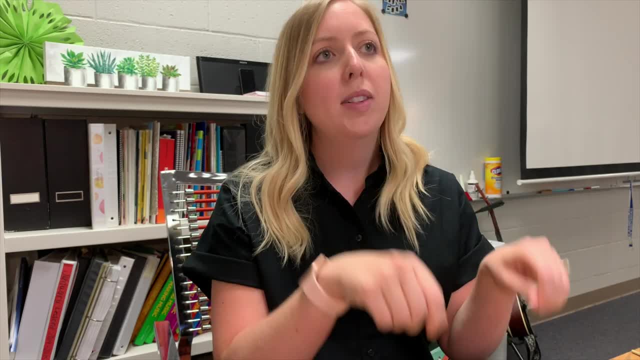 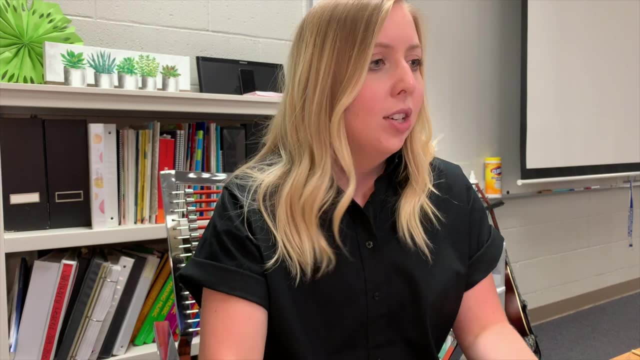 really nice job of. like the first time they just did it without a drum And once they had it, then I added in the drum beat and some groups were successful and some weren't, And so I just wanted to make sure that they're not. but that's okay. Okay, Let's talk about then. finally, second grade. second grade: I did Charlie over the. 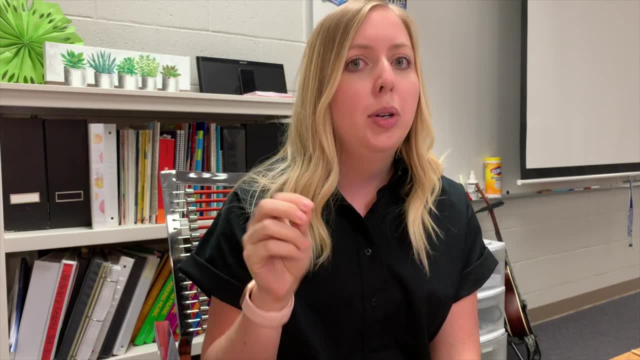 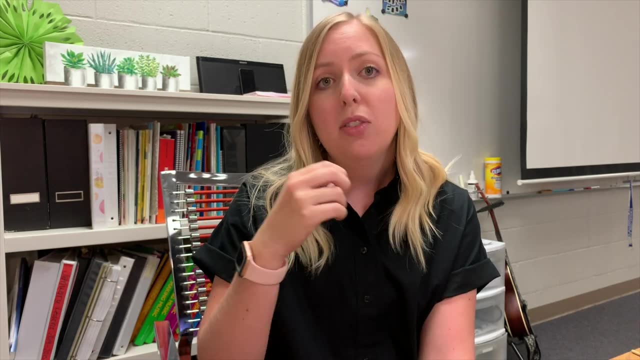 ocean classic and I am checking off as students sing by themselves. just that they did it, that you know they um, and it just a mental note like, or a little check Mark if maybe a student was really off pitch or something. 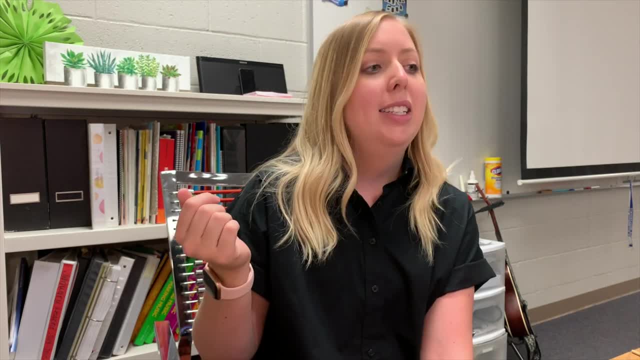 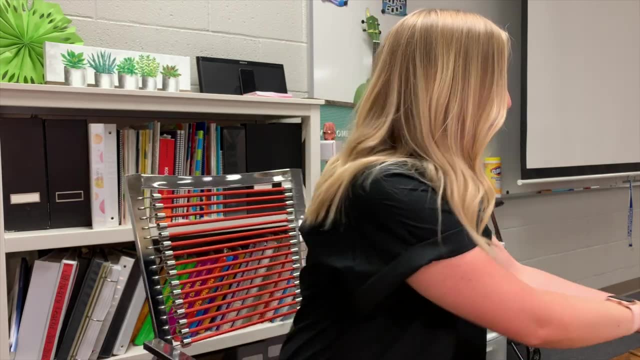 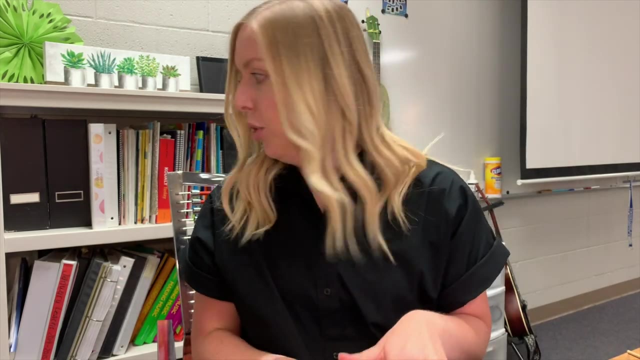 like that. just know that I need to kind of work with them a little bit more. Um, I did that, Bernie B, which actually you probably saw in my little montage. I was creating the slides for that's out of pathways. I have never used this book, Um, I have the other one too. I can't remember where it is, Um, but I am really. 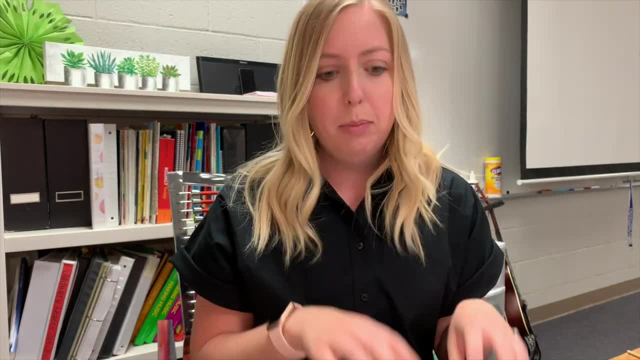 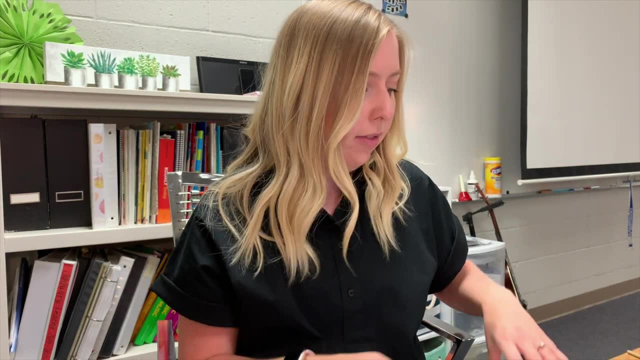 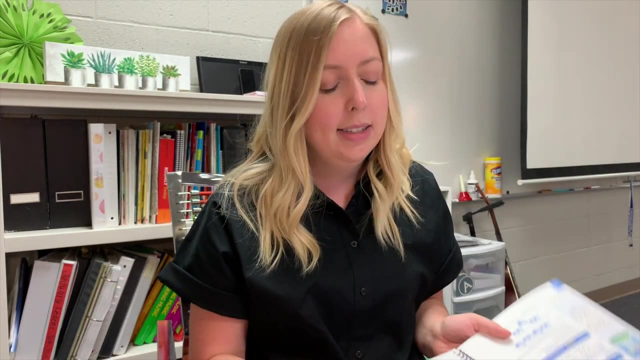 liking it so far. Again, it's kind of like an or based book um literacy, ensemble movement and improvisation and composition. So I'm using the first lesson or the second lesson out of it, Bernie B and I've really liked it so far And so pretty much the first thing was learning this rhyme and 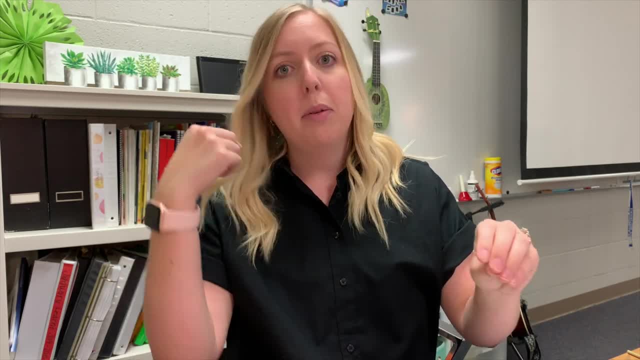 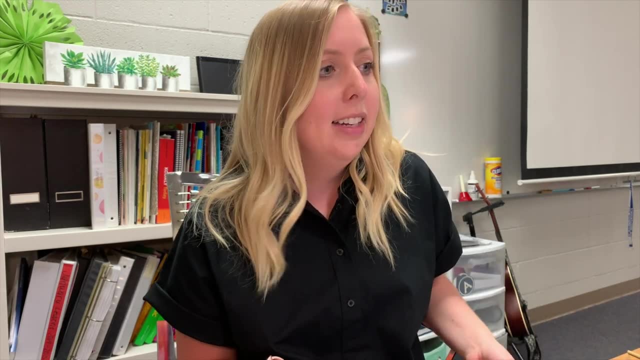 um doing beat versus uh rhythm. So there you know, we had beat on the hand drum and then Lumi sticks played the rhythm of this rhyme And I can tell my second graders especially: they need more work on what study beat is, because a lot of them. 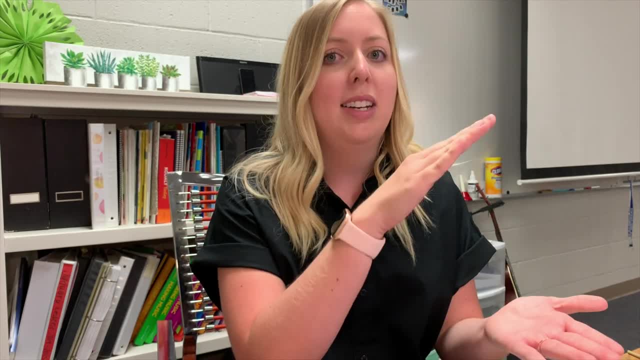 wanted to join in with the rhythm side and they couldn't quite keep that study beat. They were starting to do the rhythm, So we'll see how to go back and forth. Um, and then I did that Pokemon catch game also with them, but 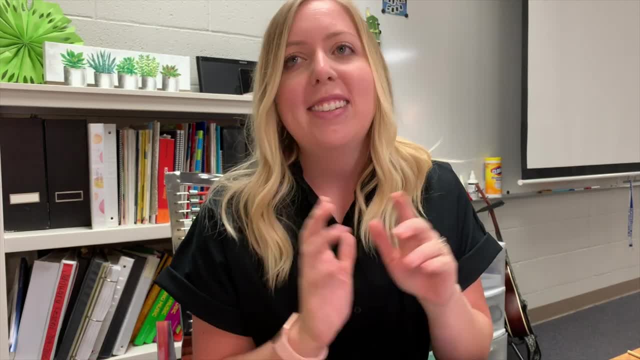 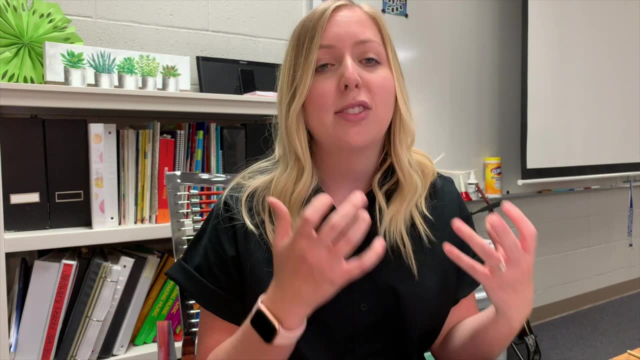 just with time TT, I wanted to do down down baby, which I think is just such a fun song. Um, I, I try and do that with first, Uh, kinder, first and second. just do those like classic songs that sometimes we don't kind of skip over if you don't have. 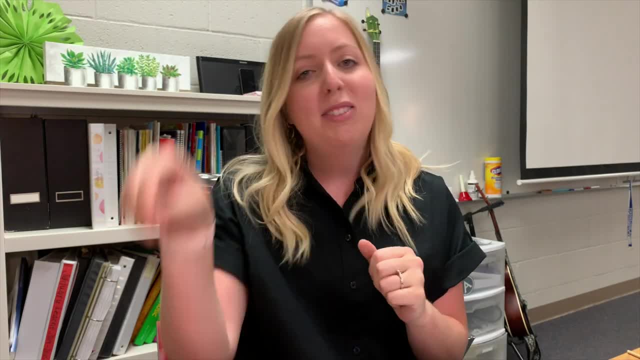 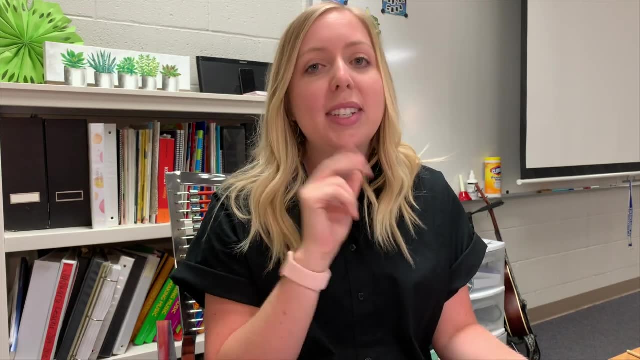 them in music. Um, but I did. I actually missed out on that, So I'll have to push that back to the next lesson. All right, So fourth, third, second down. Now I got first and kinder this afternoon, So again I'm going to kind of double. 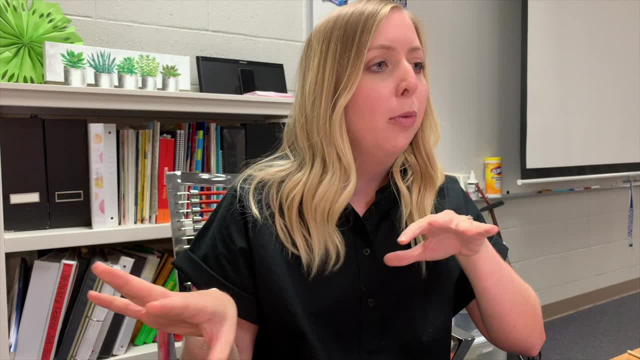 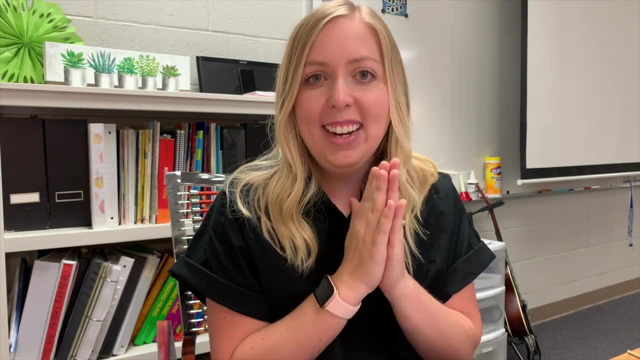 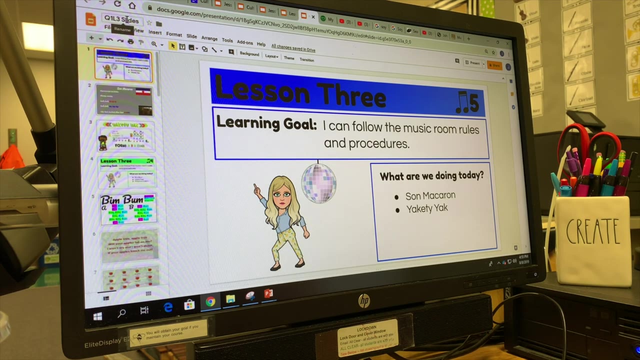 check my notes. uh, make sure I have everything ready and out for them, Cause I have no downtime in between lessons. Um, so I need to be ready and then I'm going to go to lunch. All right, Bye, guys. So here is my lesson- three slides. So I've been really loving trying to put everything into just one PowerPoint, And I love. 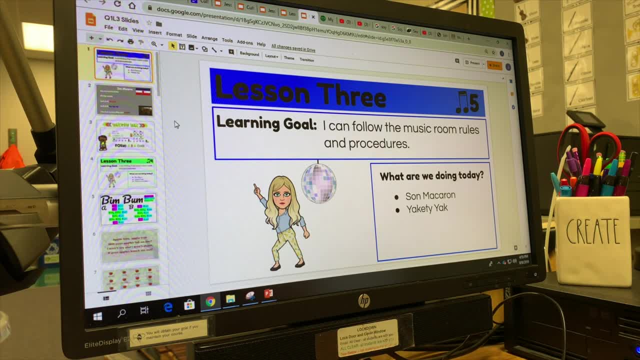 Google slides because it makes everything so easy- embedding videos and all of that. So I try and keep it all in one PowerPoint. Their learning goal is always here, So I don't need to write it anywhere, because I just show them when they first come in and 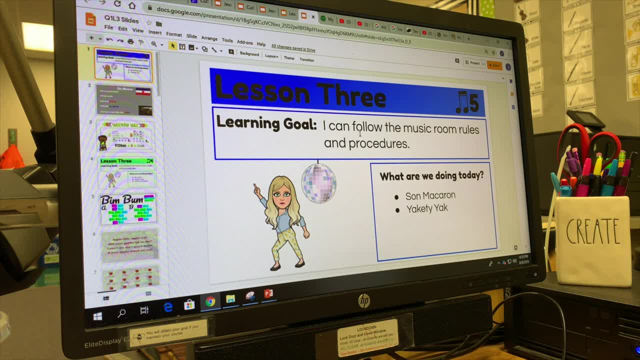 remind them about it. Um, and so I've been liking that a lot, because then I don't have to come over to my computer and click out of something. Instead, I can just use my PowerPoint clicker from anywhere and I don't have to worry about like walking over to my computer, because that's. 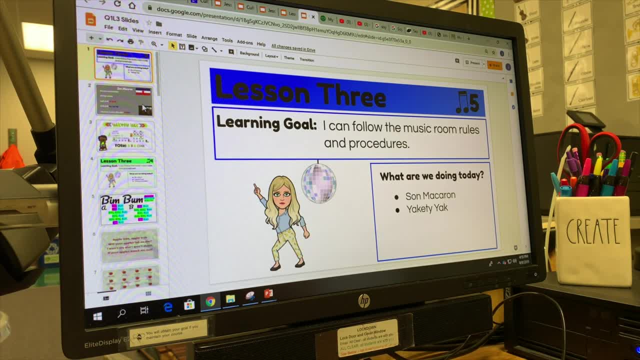 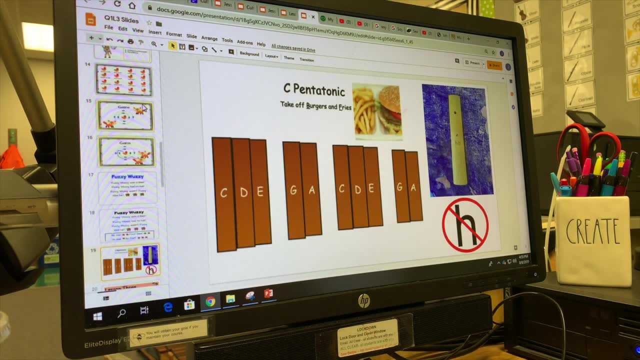 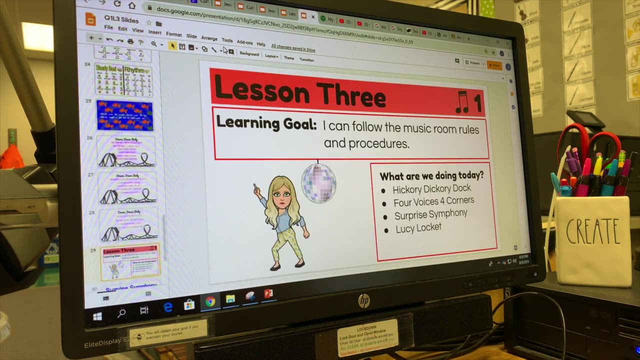 usually where I kind of start to lose them. So I'm going to go through to talk you guys through what I did with kindergarten and first grade today. So okay, So, oh, this is second grade, Let me see, Okay. 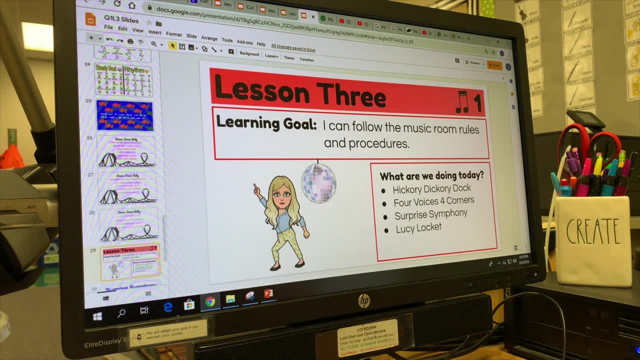 So lesson three with them. still, my learning goal for all of them is just that they can follow music room rules and procedures. Still the beginning of the year. I want them to work on that and I always put a little list of what we're doing today. 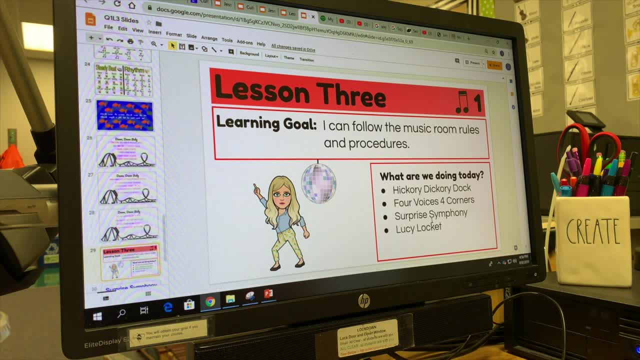 It's for them, but it's also for me to keep me on track because I can ever. if I forget, I just look up at the board and I'm like, oh yeah, that's next. So I did hickory, dickory dock. 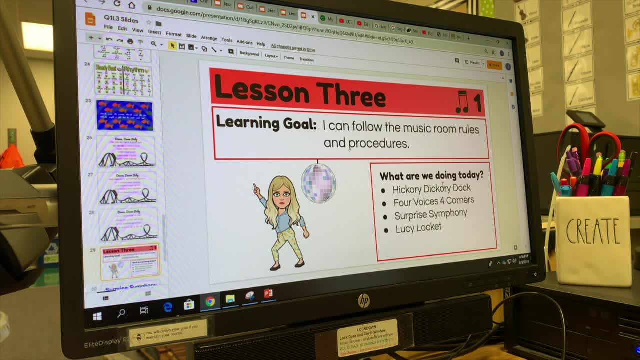 I get this is a game plan again, instrument activity. So they play the tick-tock ostinato, just steady beat tick-tock, tick-tock on wood blocks And then we say the rhyme: hickory, dickory, dock over top of it. 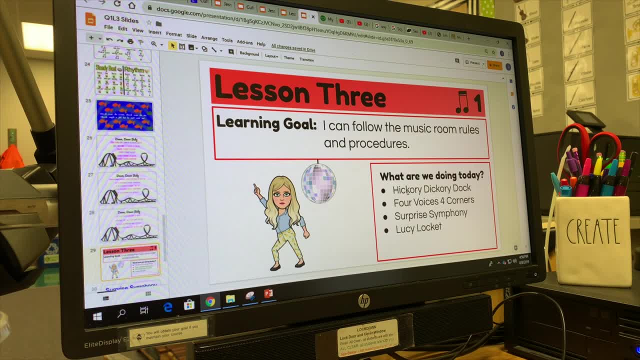 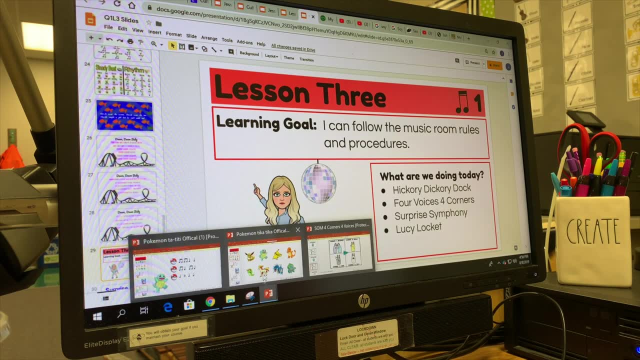 They did pretty well But again still need a lot of that study beat reinforcement. Some of them stayed with the study beat, some went a little too fast for corners. I got this from Cilio music, So she has a bunch of four corners games and they're really nice. 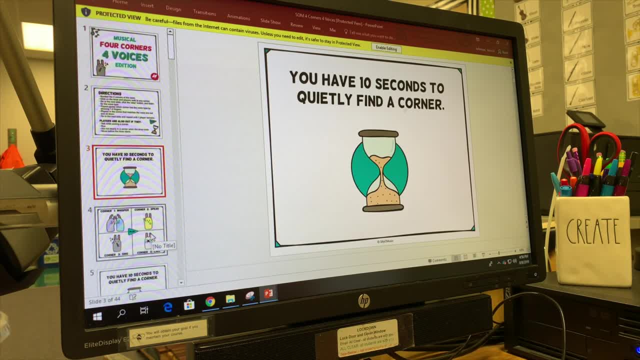 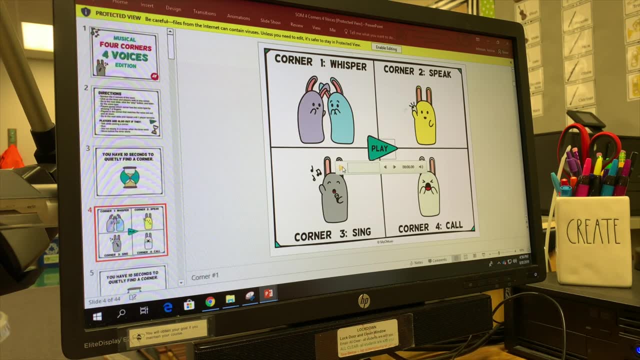 They have a 10-second countdown, So the kids go to a corner of the room. I press play and it does the four voices. So, like this one, see if you can hear that it was whispering. So the whisper corner opens. Whoops. 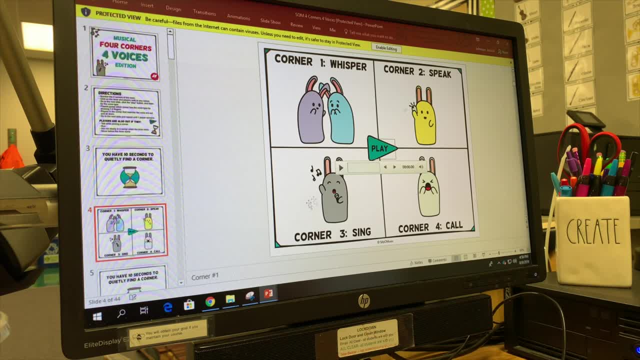 The whisper corner would have been out, And so they would go set up their spot and then we would go again. They would all pick a corner in the room. I would do the 10-second counter and then I press play on this again. 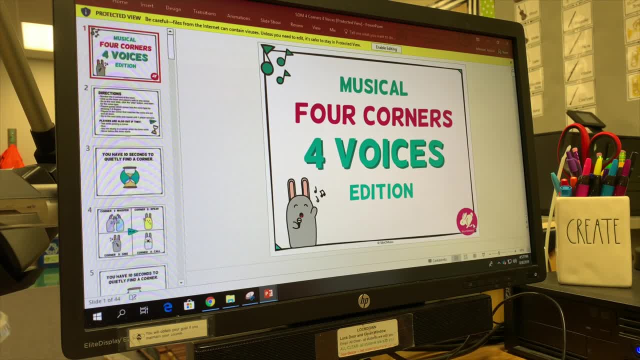 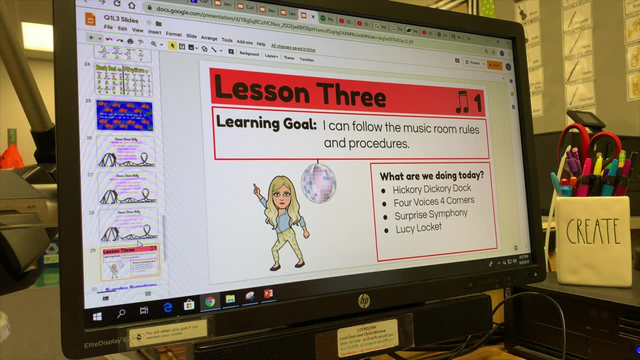 And so it's by again, Cilio music. So I like these a lot. I have quite a few of them. So a good review for kindergarten or from kindergarten. Then I did the surprise Symphony, which I just did. this They all said he looked like George Washington. 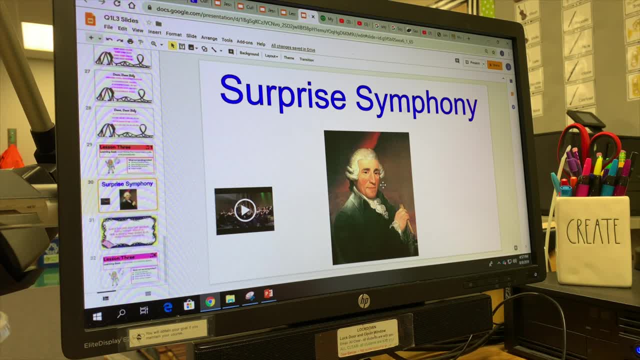 We talked about why Haydn would have, you know, a wig on And that was the fashion. And then I tell, always tell them the story. And there's been so many different lessons, lessons available on this, But my kind of version of the story is that Haydn was asked to go to a king's house and do some music for him as palace. 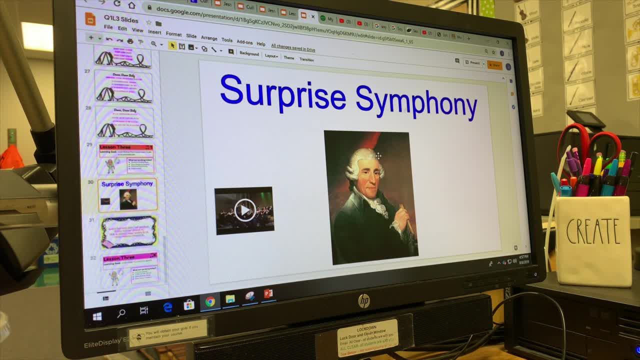 And he worked on it for months and months and months And he was going to do the symphony and he practiced with the orchestra And he finally does the concert and he looks back And if you have ever heard this music Like, it's very, very like soft and lullaby ish in the beginning. 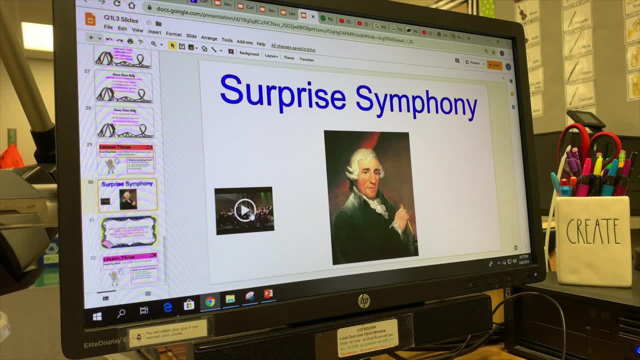 And so I tell them that Haydn looked back because he just couldn't wait to see the king's face and just how awesome it was. And he looked back and the king was asleep and he couldn't believe it. So he decided to wake up the king by making a forte music, because we're doing a little bit of review on piano and forte. 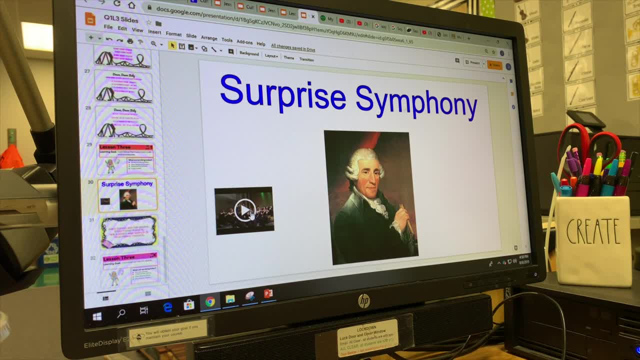 So I talked about like we. he woke him up. Haydn was sneaky and did a forte move or a forte conducting gesture And made the orchestra play forte, And it woke up the king and surprised him. And then we reenact that. 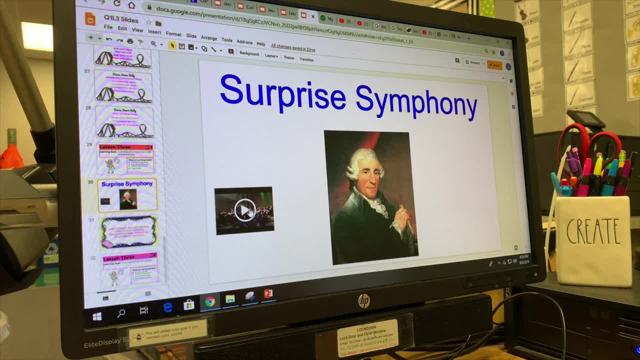 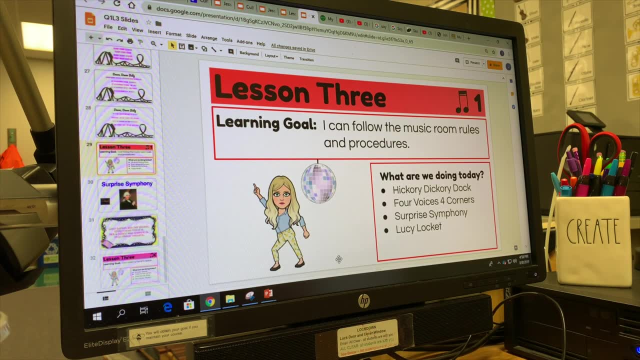 So I tell them the story, I play it for them, And then we play it again, And this time they reenact being the king. And then I actually ran out of time for Lucy Lockett, But again another. I'm doing loud and soft right now. review. 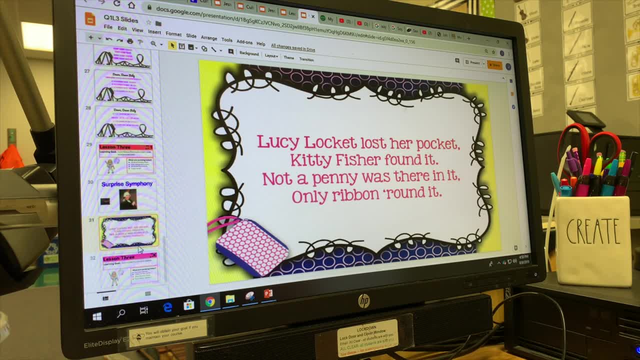 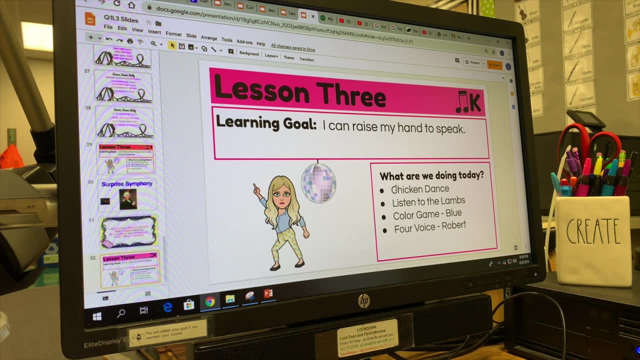 So I was going to have them play that, because they played it last year. But no worries, We ran out of time, But they've already done it, So that's all good. Then for kindergarten we did the chicken dance. So if you use game plan again, 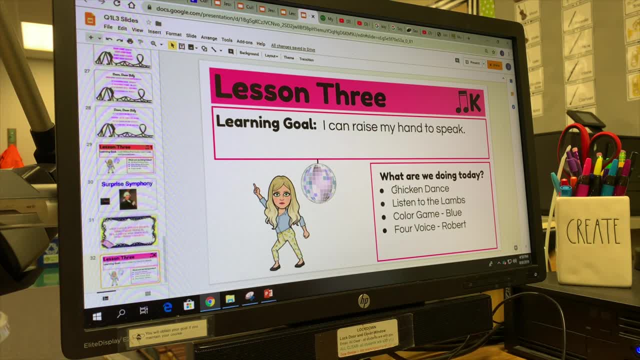 Can you tell I like game plan. If you use it then you know that kindergarten in the beginning you're going down to the farm, Every single lesson has a certain animal And that certain animal correlates with a certain instrument, like non percussion. So pretty much in the beginning like it's the ducks. 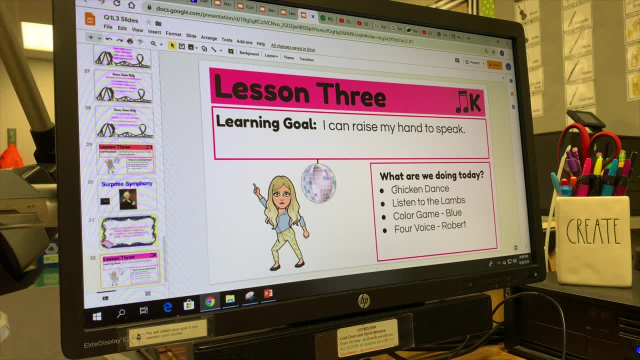 The ducks play the loomy sticks, Then chicken They play the tambourine, And then I also had the lambs today which play maracas So slowly. every day I introduce a new instrument, Animal, We do animal kind of themed and other songs or games that I have with them.